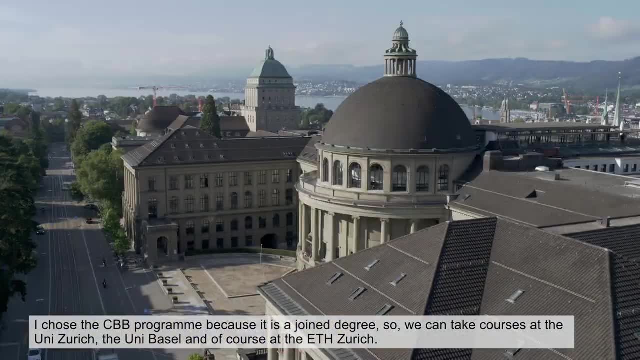 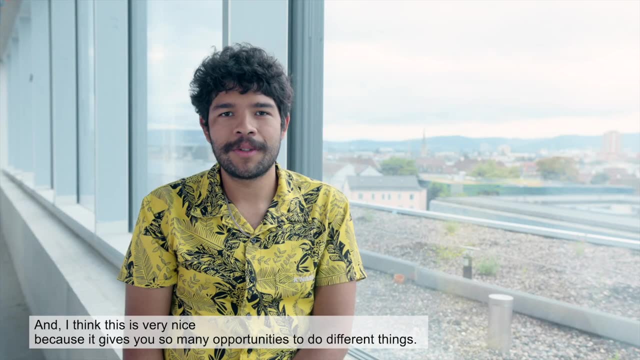 because it is a joint degree, so we can take courses in the Uni-ZURI, we can take courses in the Uni-Basel And, of course, in the ETH Zurich, And I think this is very nice because it gives you so many opportunities to do different things. 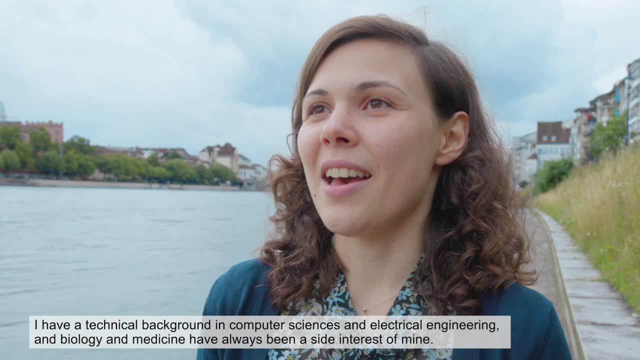 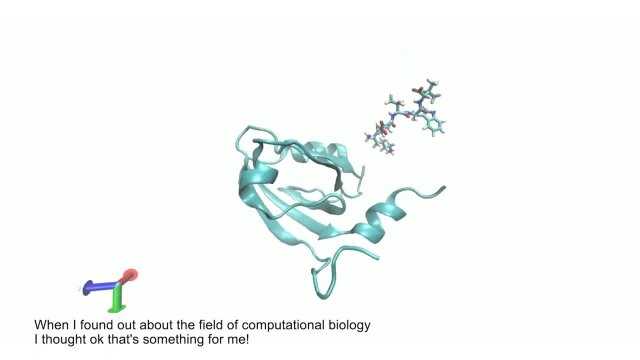 I have a technical background in computer science and electrical engineering, and biology and medicine has always been a side interest of mine. So then when I found out about the field of computational biology, I thought, okay, that's something for me. It really matched my interests at that point and it still does. yes, 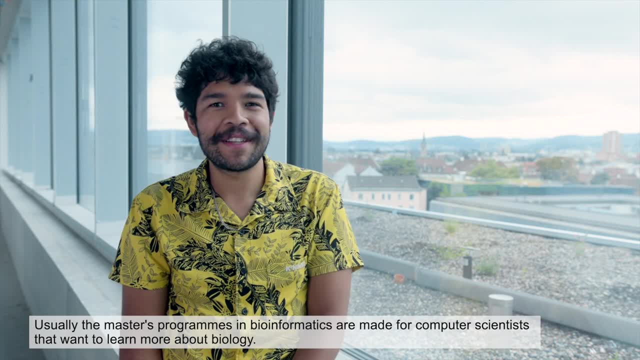 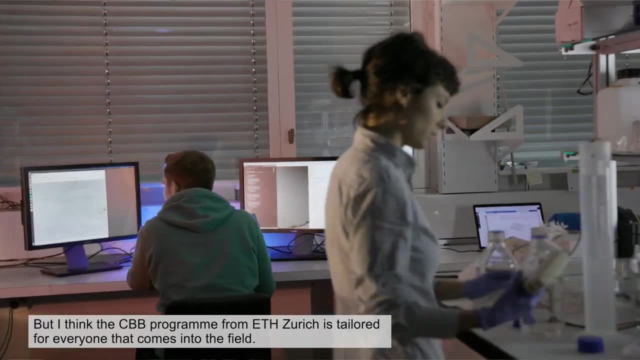 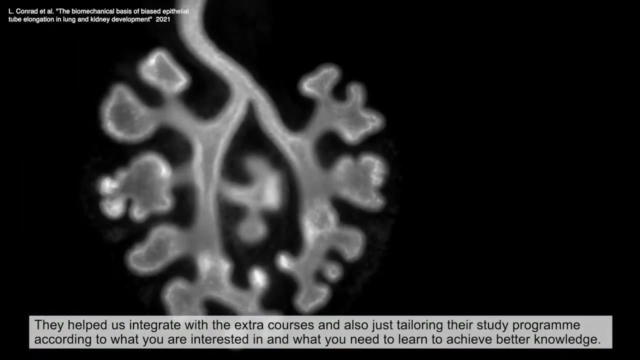 Usually the master programs in bioinformatics are made for computer scientists that want to learn more about biology, But I think the CBB program from ETH Zurich- it is tailored for everyone that comes into the field. They helped us integrate with the extra courses and also just tailor the study. 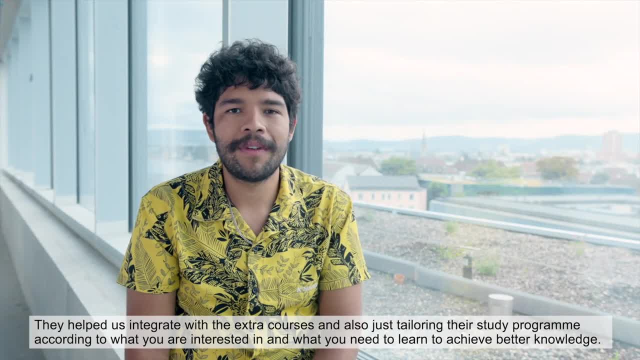 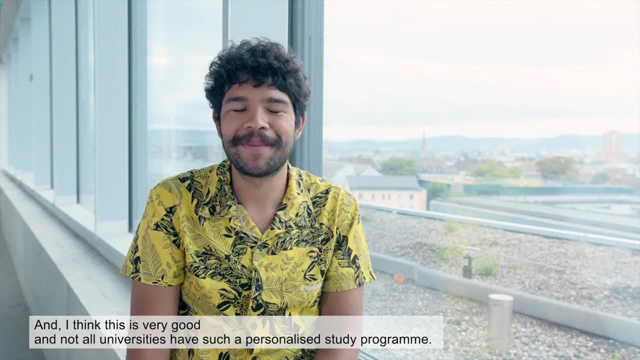 program according to what you're interested in and what you need to learn to achieve better knowledge, And I think this is very good, and it's not only universities that have such a personalized study program. There is a mentor system. So at the beginning of the program, in the first six months, it's 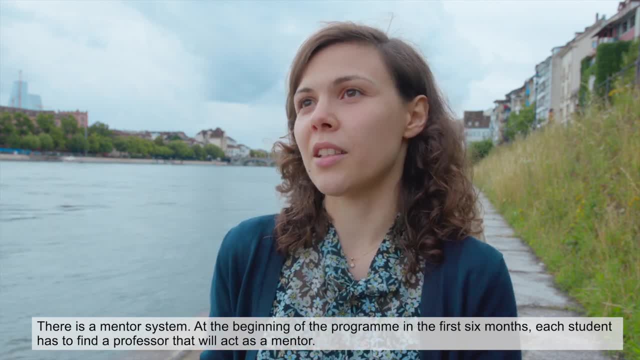 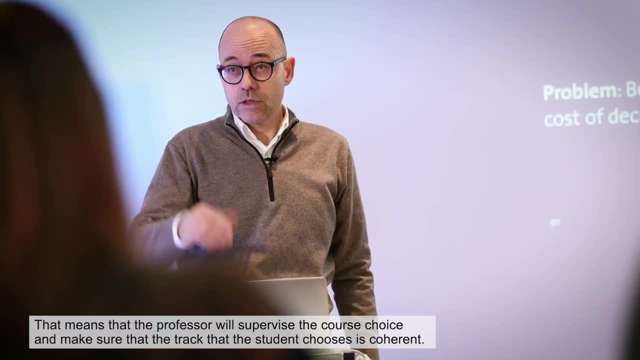 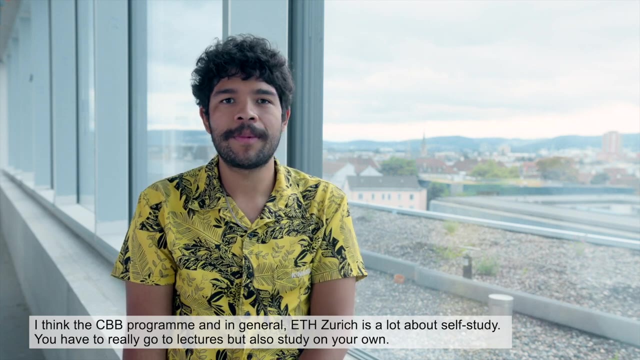 Each student has to find a professor that will act as a mentor. That means the professor will supervise the course choice and make sure that the track that the student chooses is coherent. I think the CBP program and, in general, ETH it is a lot about self-study. 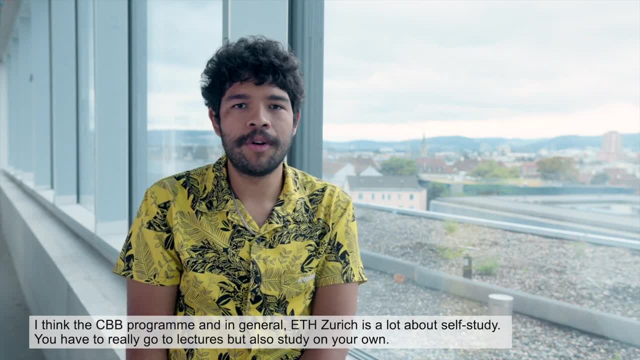 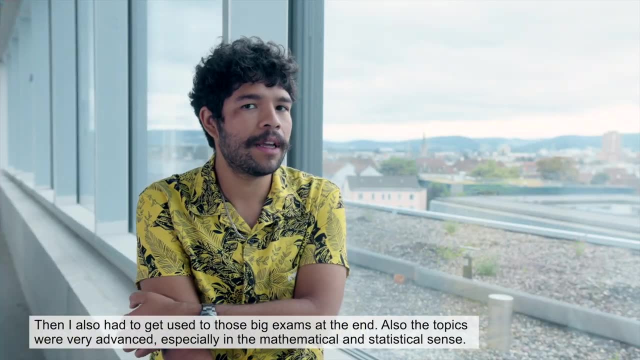 You have to really like go to lectures but also like study on your own, Then I also had to get used to these big exams at the end. So the topics were very advanced, I feel like, especially also in the mathematical and the statistical sense. 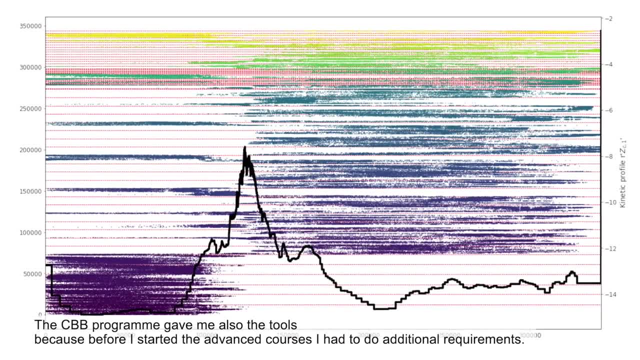 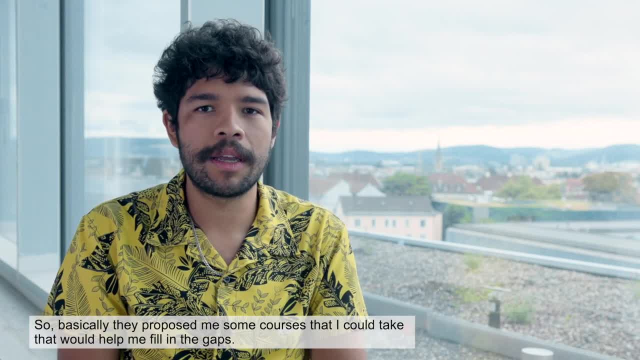 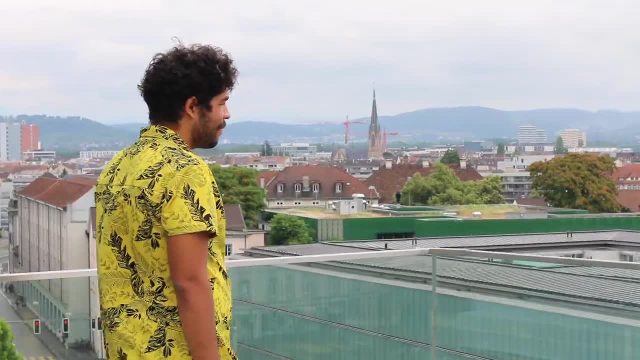 The CBP program gave me also the tools, because before I started the advanced courses I had to do additional requirements. So basically they proposed me some courses that I could take that would help me fill in the gaps. So before starting the program I saw that the department was the Biosystem Science and 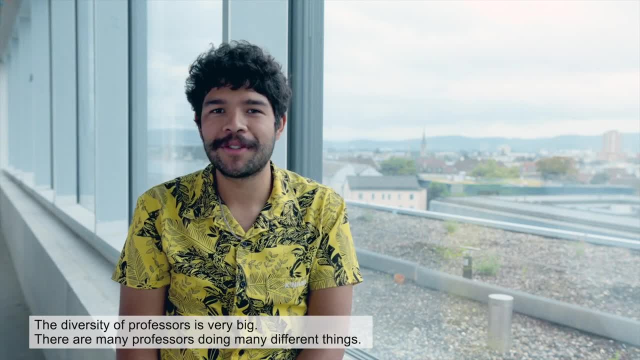 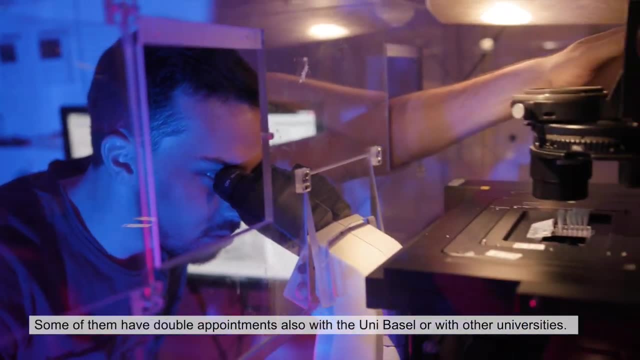 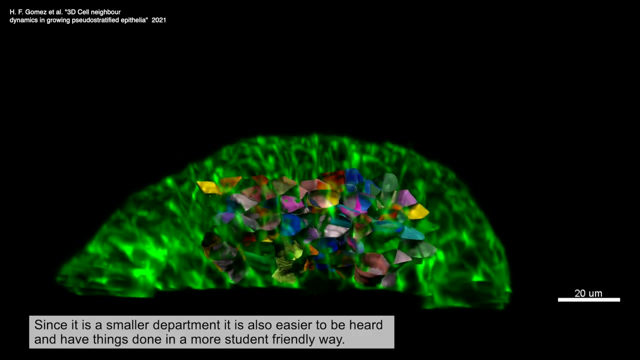 Engineering Department, The DB, The diversity of professors is very big. There are many professors doing many different things. Some of them have double appointments, also in the Unibus and in other universities. This I found exciting because for men's collaboration, since it was a smaller department, it is also